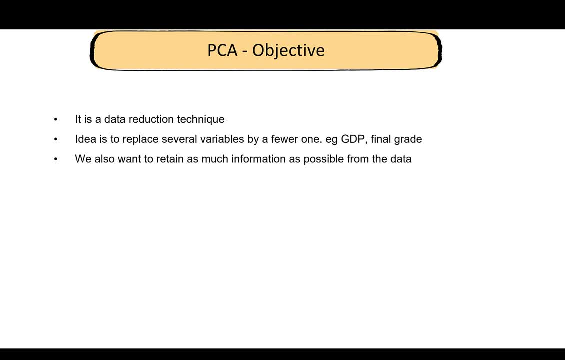 So we want to retain as much information as possible from the data. That makes sense, right? So what do I mean by information? Information in the data basically means variability in the data. I don't want to use the variation or the variability in my data set when I reduce the number of variables. 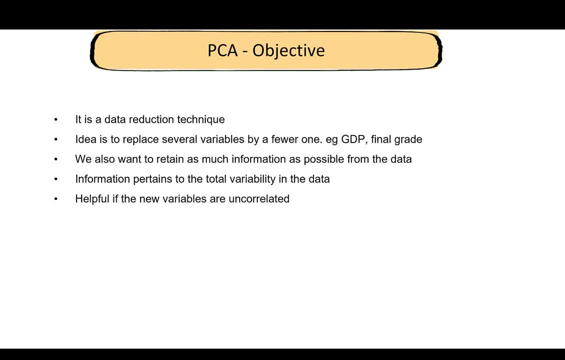 And it is also helpful if the new variables are uncorrelated, right? So if you think of statistical techniques like regression, if your predictor variables are highly correlated, you will run into issues. You will run into issues while implementing regression. However, if your variables are uncorrelated, then things run pretty smoothly, right? 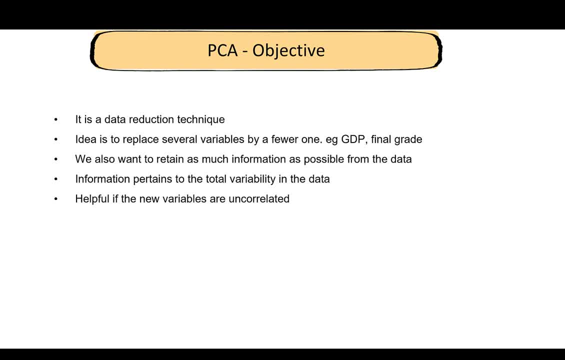 So PCA can help us implement, or these variables that are obtained from this PCA technique can help us run some of the other statistical techniques smoothly. So, to summarize, PCA aims to reduce the dimension of the data. When it does so, it wants to retain as much data as possible. 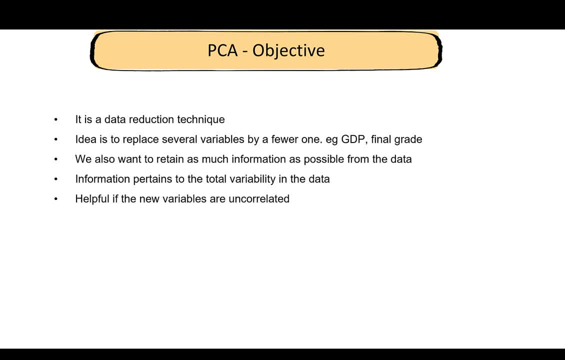 It wants to retain as much information as possible. Retaining information is the same as retaining or maximizing the variability in your data, And we want the variables to be, or the new variables to be, uncorrelated. So let's see, how can we, how can we look at this more mathematically? 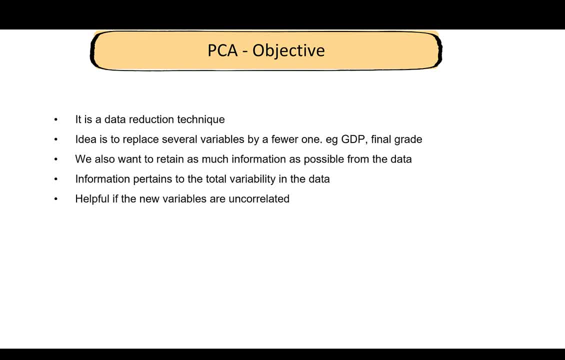 Or in other words, let's see what is the big idea, right. What is the idea, The idea behind PCA? So say, you have a study where you want to that involves P variables. So this random vector, X has P dimensions. So Y1 basically is a linear combination of your P variables. 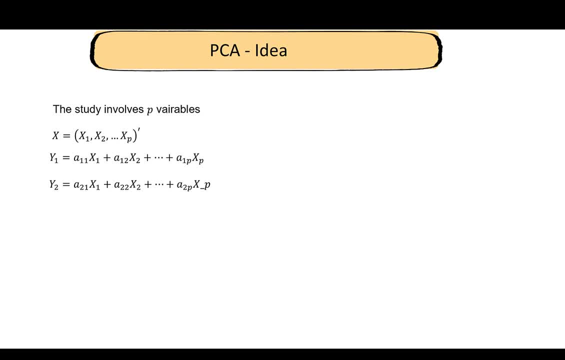 Y2 is a different linear combination of your P variables, And so on until YP is another linear combination, is a new peak, is a new combination of your P variables. so y1, y2, yp, right, we have P new variables which are linear combinations of your original P. 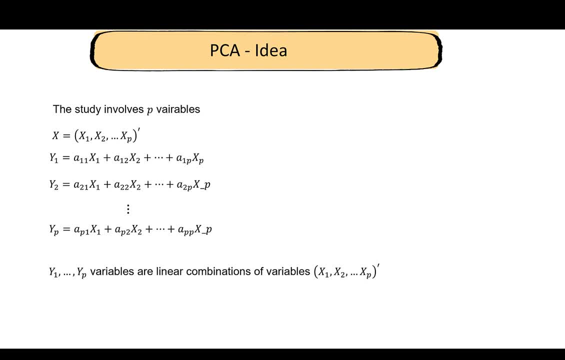 variables. so at this point you might be wondering: right, we have P variables x1 through XP- that are the original ones and we have new P variables, which is y1 to yp. right, how are we reducing the dimensions? right, we still have P new variables. so what is the point of this? that's a legitimate question and we, and 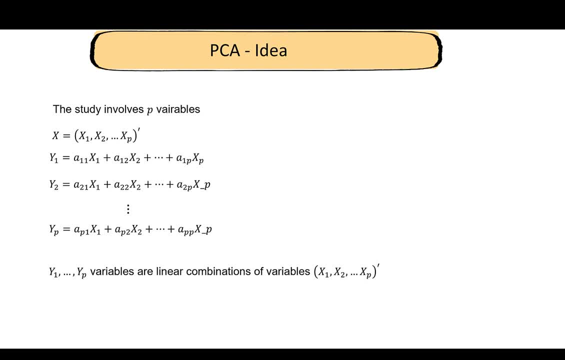 I'll get back to it later on. so just for convenience, we are going to think of y1. we are going to write it as a1 transpose X, where a1 contains all of the constants or these coefficients of the linear combination, a2 contains all of the constants for y2 and ap contains all. 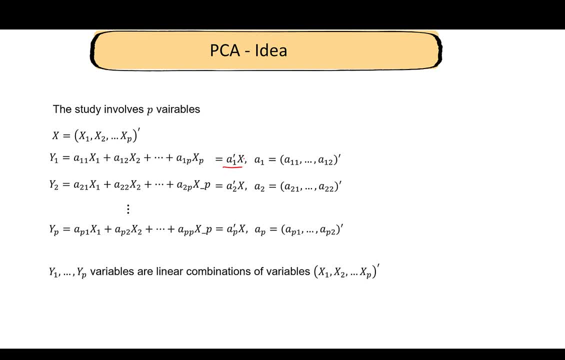 of the constants for yp right. so yp is basically nothing but a P transpose X. so it's a good idea to keep a note or track of all of these notations, and we will be using lot of vectors and matrix matrices in this course and this and 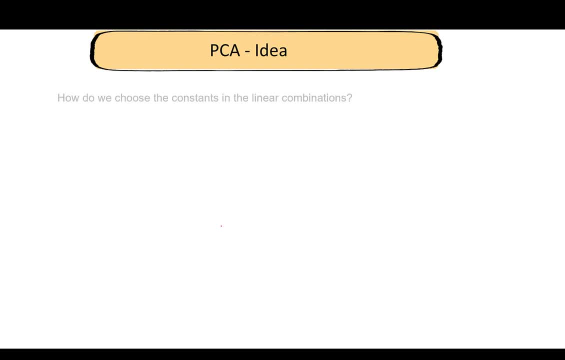 especially in Pca. so how do we choose all of these linear combinations? right, so remember our goal: reduced dimension, retained variability. and we want uncorrelated variables, right so we want to choose all of these constants such that these three conditions are satisfied. so let's see so. 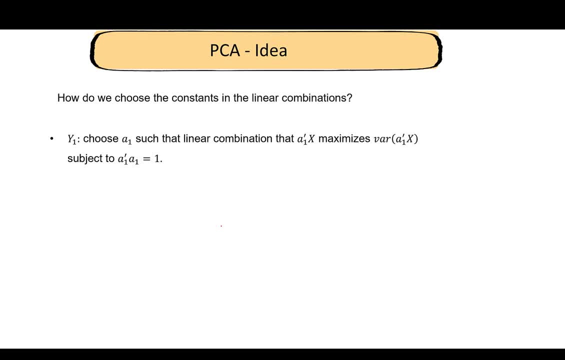 for y1, we want to choose a1, and we want to set this P, transpose X as 0 for one of the data variables, and we want Including variables' that are from one, a1,. so if we study this record of 2'000acci too, all of these variables are missing, And so we see. 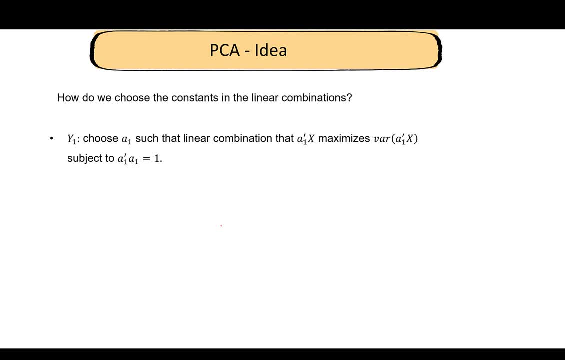 right to retain the variability or the information. so basically we want to find the constants that maximize this variance. so we want a1 to maximize this variance of a1. transpose x. think about a random variable for a second. any random variable, say right. and if you multiply that random variable by 10, right. so variability of um, say your variable is w. so 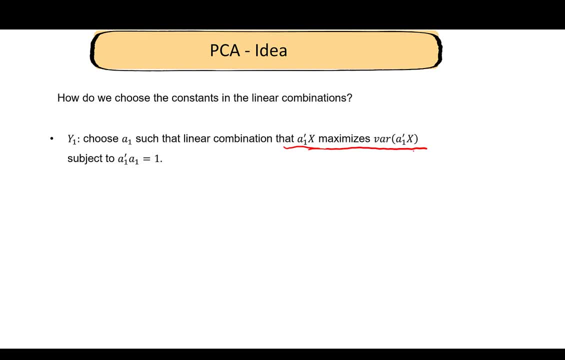 variance of 10 times w is greater than variance of w. variance of 100 times w is greater than variance of w. variance of million times w is greater than variance of 100 times w. so what i'm trying to say is: i can, or we can, keep on increasing variance by taking 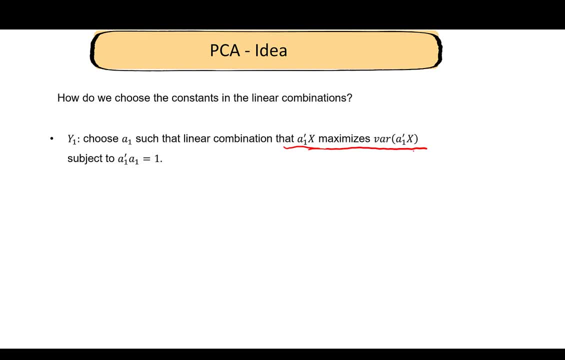 larger values for a. but we don't want to do that. that is not very informative. so we are going to put this additional constraint. we want to choose these constants such that this: a1 transpose a1 or norm of the vector, a1 is 1, right, so this stops us from artificially inflating the variance. so 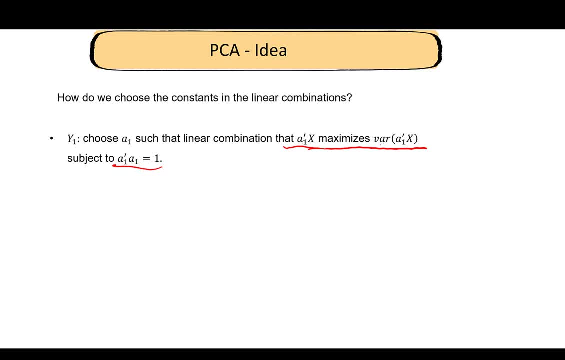 y1 is such that variance is maximized, and it satisfies this condition. and y1 is maximized, and it satisfies this condition. and y1 is the first principal component. y2 again, we choose a2. right, we choose this vector a2, such that the linear combination has maximum variance, subject to this condition, that norm of a2. 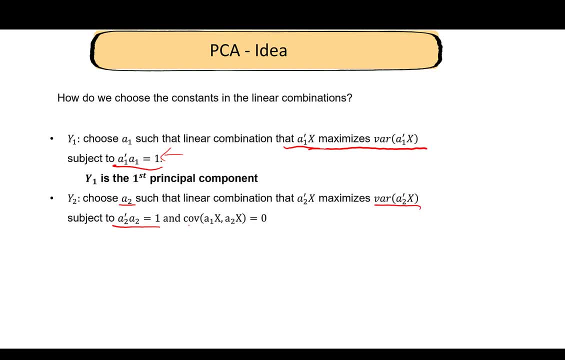 is 1 an additional condition, now that a2 or sorry, additional condition- that a1 x and a2 x. this should be transpose here. and then we have a1 x and a2 x. this should be transpose here, right? a 1 transpose x and a2 transpose x is equal to 0, that is, y1 and y2 are. 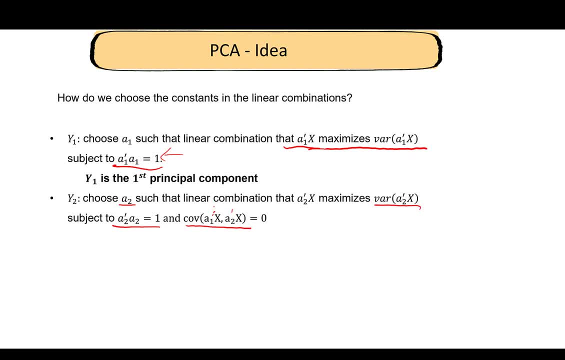 uncorrelated in general, Oh and y2 is the second principal component. so in general- for I write- we choose this vector a, I to maximize the variance of this linear combination, which is subject to this condition that the norm of vector ai is 1 and yi is uncorrelated with all of the 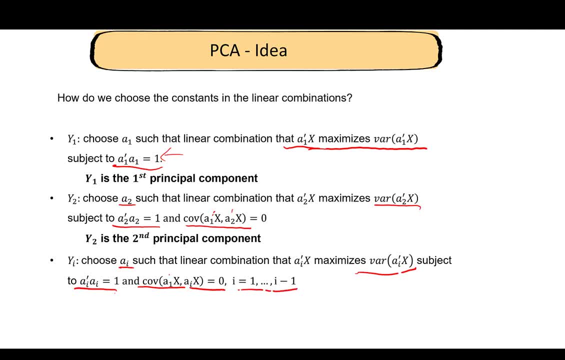 previous principal components. right, so covariance of a1 transpose x and ai transpose x is 0 for i, going from 1 to i minus 1. so yi is uncorrelated with all of the previous principal components and yi is the ith principal component. so you can see that we're constructing these new variables, which are basically the principal. 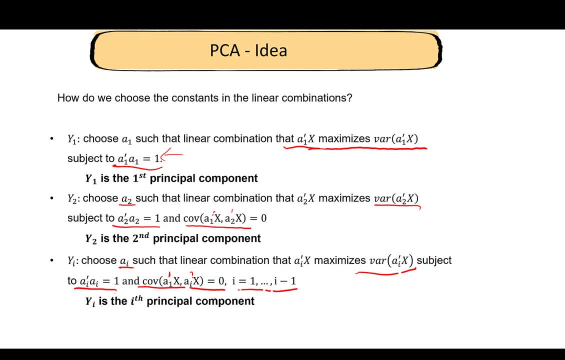 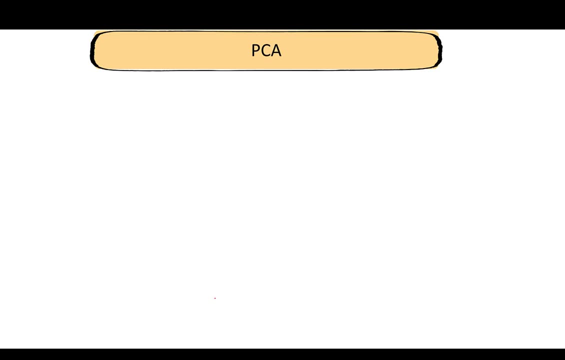 components such that they maximize the variance in some sense and they're uncorrelated with each other. so two of the three objectives right that i mentioned are satisfied here. so okay. so how do we get the dimension reduction right? we still have those p principal components, right. so, in general, if our data has p variables, we typically need 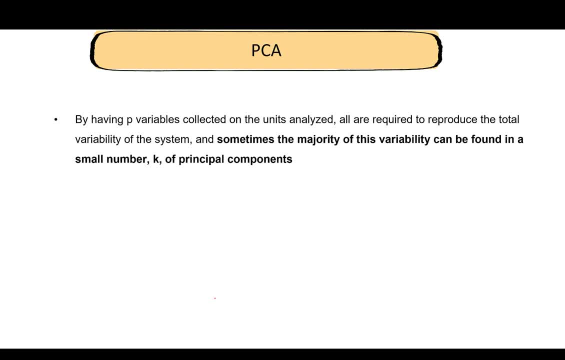 p principal components or all the principal components to reproduce the total variability of the system. however, sometimes it's possible that majority of the variability can be found in a smaller number of components. so suppose you have 20 variables right and you do the, you calculate the principal components and it turns out that the first three principal components 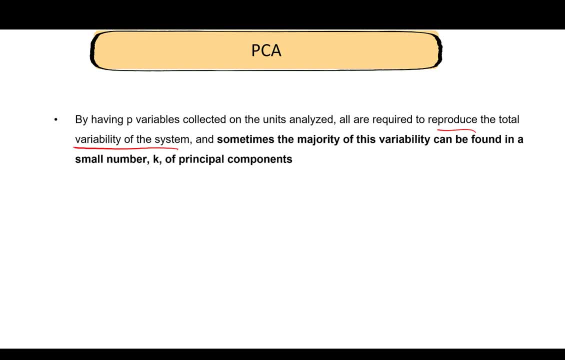 amount for 99 percent of variability. so in this case, instead of looking at all the 20 variables, you will consider only the first three principal components. so this is what is meant by data reduction. remember, the first three principal components are the small linear combinations of all of your 20 variables. 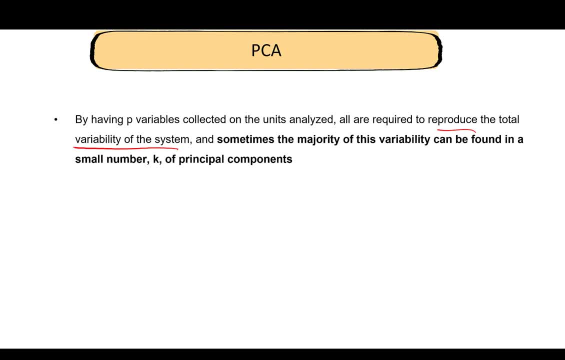 so all of this will make much more sense when we actually work with actual problems. so, if you think of a large rectangular plate, right, a plate is typically a three-dimensional object, so it has three dimensions. uh, however, for all practical purposes, you can think of, uh, think of the plate as a nice three-dimensional object. 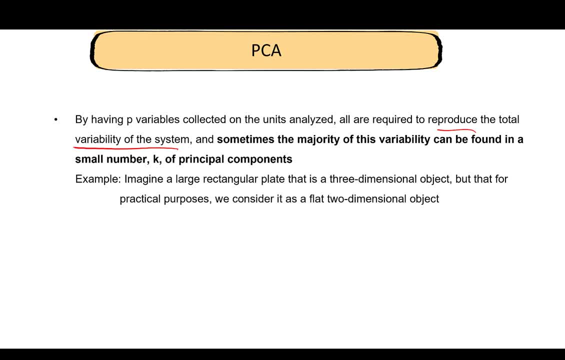 as a two-dimensional object, right? there's not nothing much lost if you think of it as a flat, as a completely flat object. so PCA is attempting to represent your data in a space that has fewer dimensions, right? so originally the data had P dimensions, it was in a P dimensional space and when, and maybe the